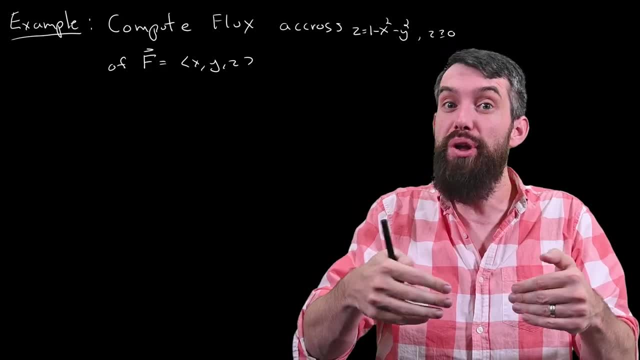 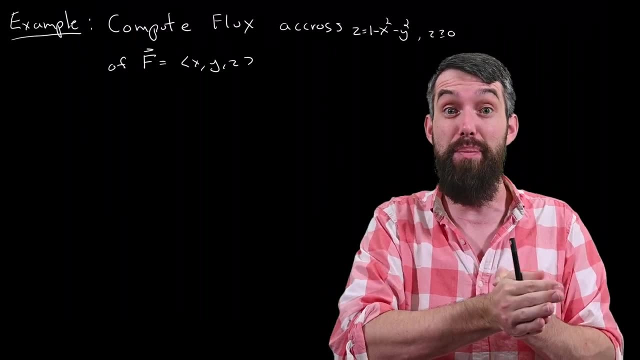 In this video we're going to compute the flux of a vector field across some surface. This is an example of a methodology that we introduced, actually, in the previous video in my playlist on vector calculus. The link to that is down in the description. So in this video we're just 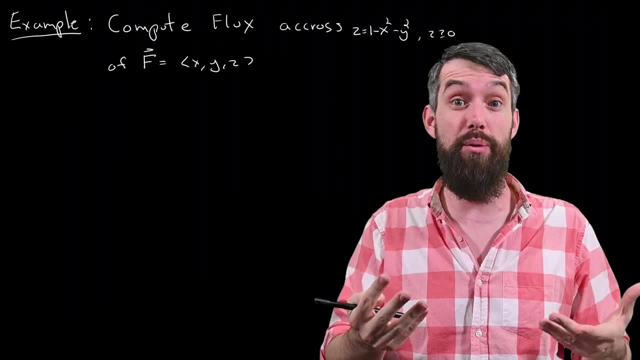 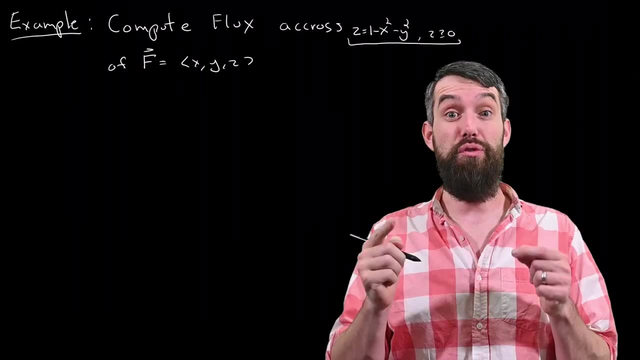 going to have the formula that we came up with previously and we're going to try to evaluate it in this specific example. So the first thing I want to do is investigate what this surface actually is. This is the surface: z is 1 minus x squared, minus y squared, and z is also greater than or. 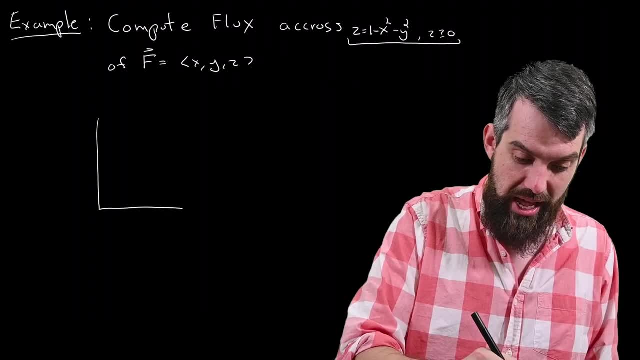 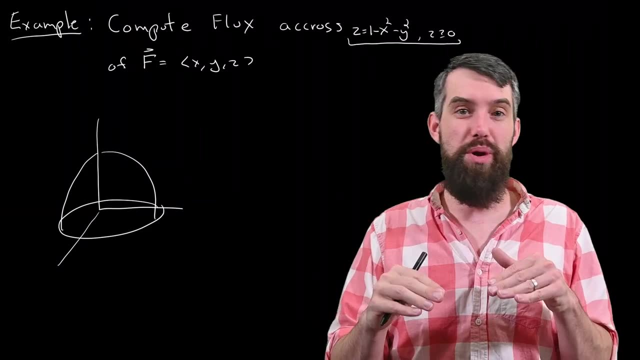 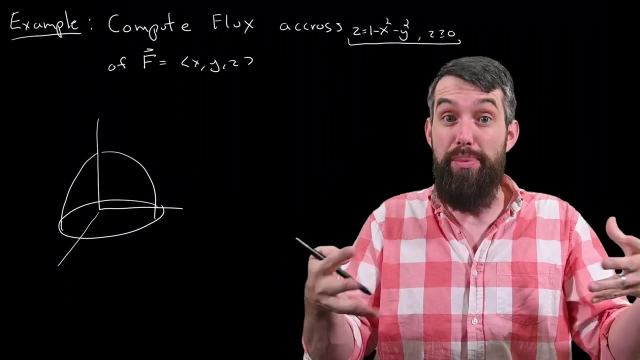 equal to zero. So graphically what this looks like is a surface that is just a parabola In the xy plane, as in: when you substitute in z equal to zero, you just get the equation of a circle: 1 is equal to x squared plus y squared, and then it looks like a parabola over top of that. 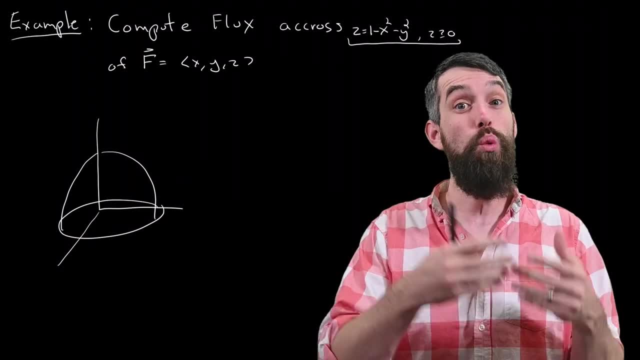 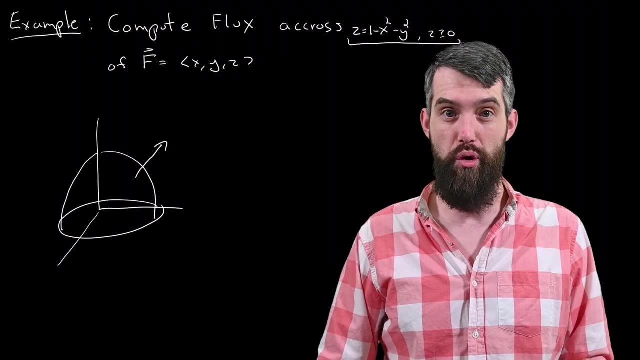 Now the only thing I have to specify, which I haven't described in the problem itself, is: which way am I oriented? I'm going to assert for you that I am ordering it with outward normals, outward, from the perspective of starting at the origin and going out through the surface. this way, I could have 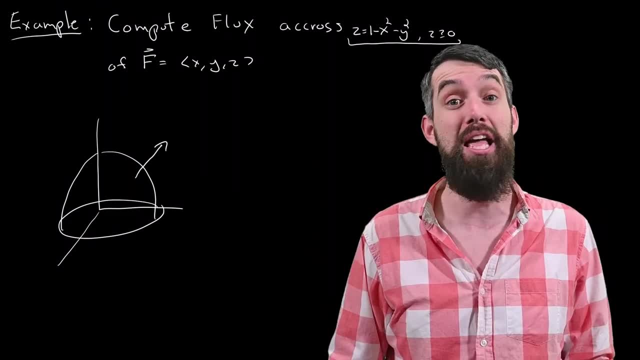 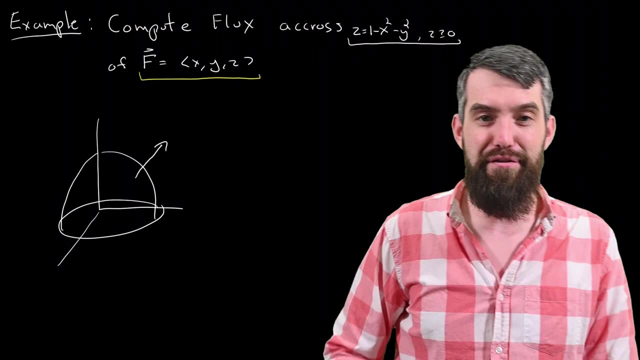 asked similarly: what was the flux going the opposite direction? But I'm going to specify, this is the interpretation that I mean. So that's the surface. And then I also have a field here, which is the field f is x in the i hat, y in the j hat and z in the k hat. And this vector field, 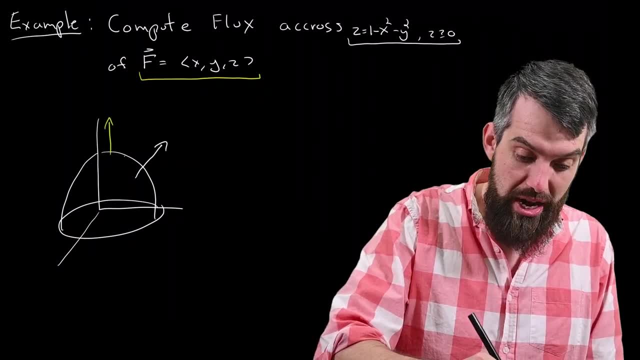 is actually one that we've seen before. This is a vector field that just goes straight out into the surface, And this is the vector field that goes straight out into the surface, And this at any point. for example, we had previously called that vector a normal vector, but it also. 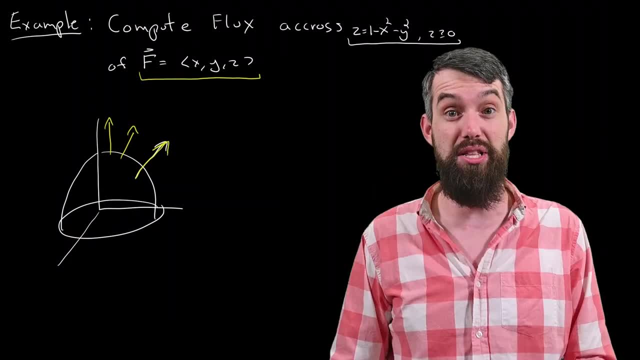 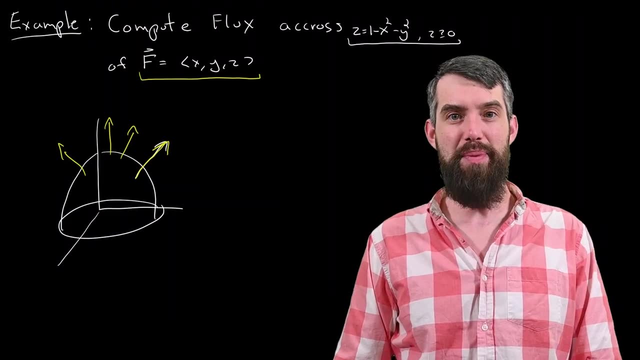 happens to be that the field vector is exactly parallel to this normal vector, So I have that sticking straight out in every single spot. Okay, so that's most of my setup. And then, finally, what's the formula I'm going to use? Well, the formula that I will use that. we spent some time. 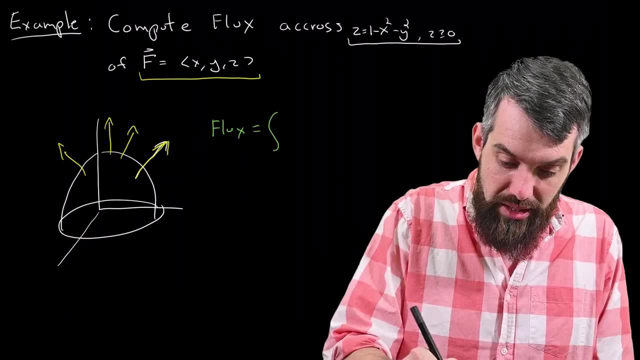 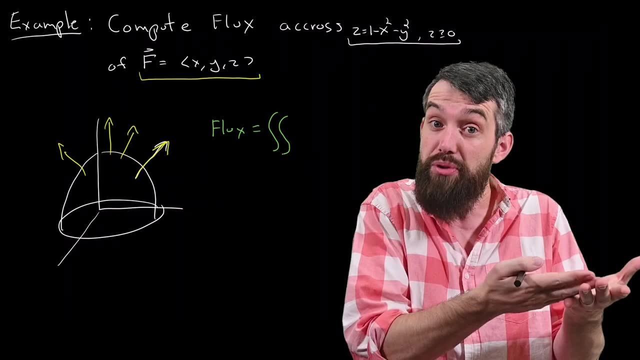 deriving in our previous video is that the flux is the double integral. And now I have a bit of a choice, because it depends on whether I want to consider the flux as a double integral or flux formula for a surface described parametrically or explicitly or implicitly, And in this case 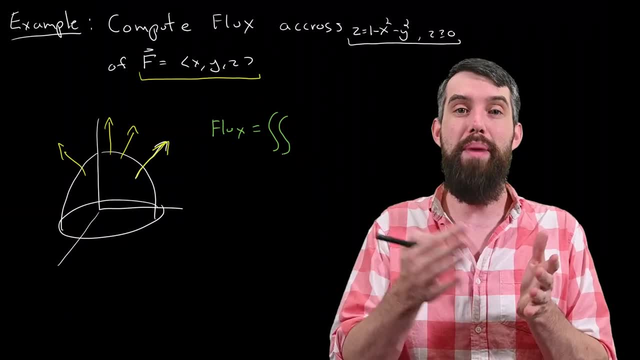 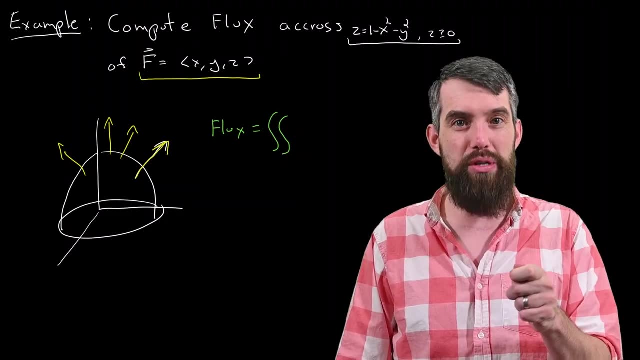 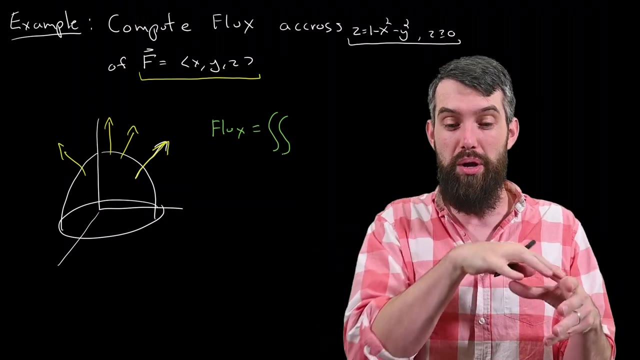 my surface actually is described explicitly: z is 1 minus x squared minus y squared, So I could use that, But the region that is imposed by z equal to 0 is a circle down in the xy plane, And this is going to be described very nicely. parametrically It's easy to describe a circle, And so, because of 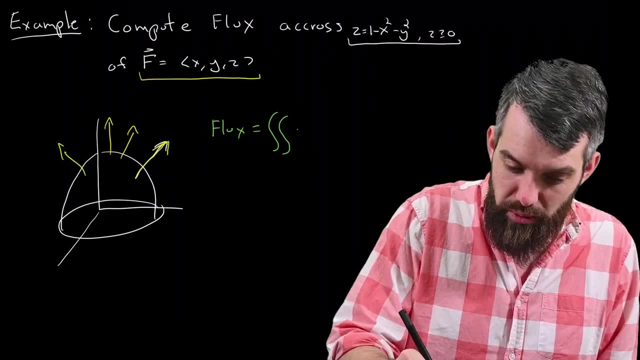 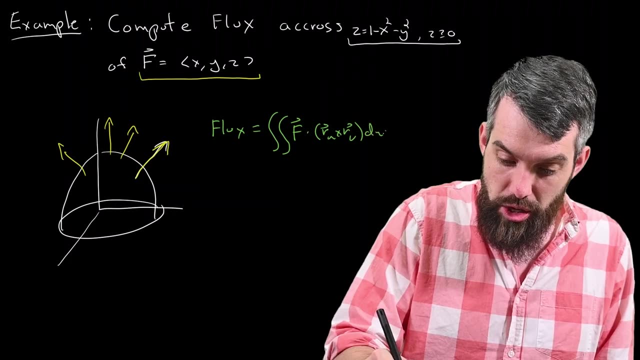 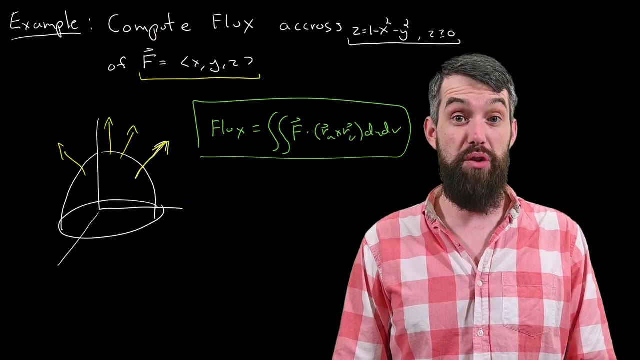 that boundary condition, I'm going to use the parametric form, in which case the integral is f, dotted with r? u, cross, r, v, du, d, v. That's the formula that we have to describe the flux, And so, really, what my goal is to figure out. well, what is this position function in terms of the 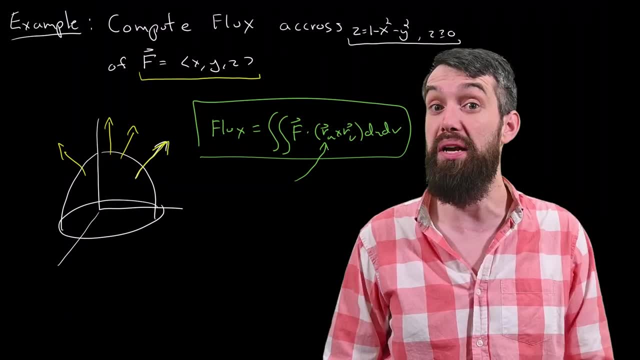 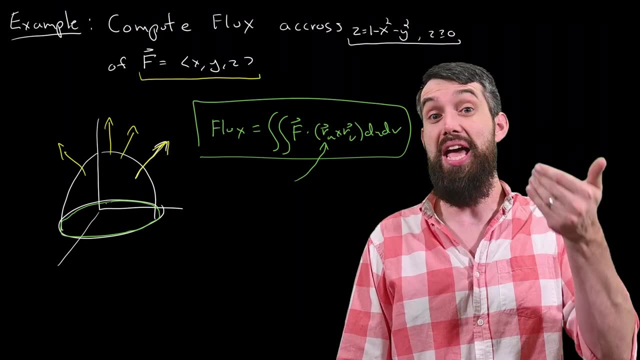 parameters u and v. What parameters should I use? If I know that, then I can more or less plug into this formula. As noted in the xy plane, we're going to have this circular region, And so r and theta inspired by z are going to be equal to z squared, And so I'm going to use this circular region. 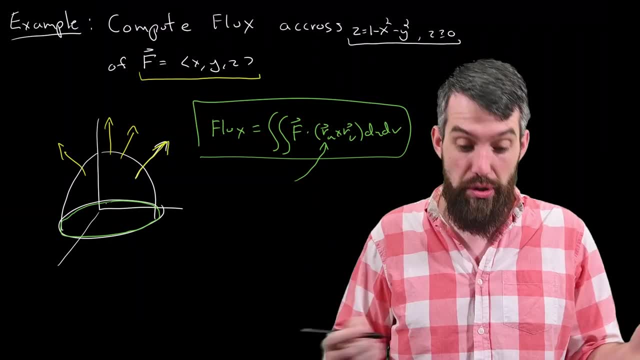 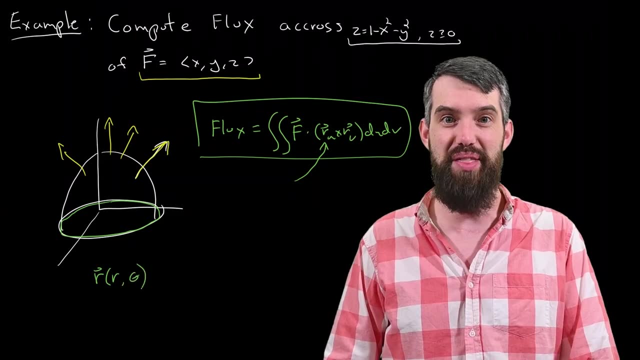 So if I do that, then my r of little r and theta. so I've got one, a vector, a position vector, and then the other, the parameter r is going to be given by. well, the x component is r, cosine of. 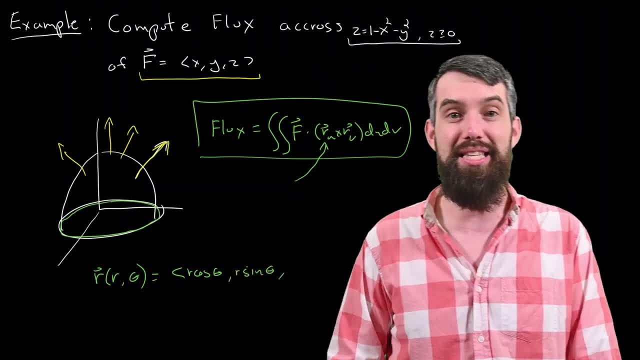 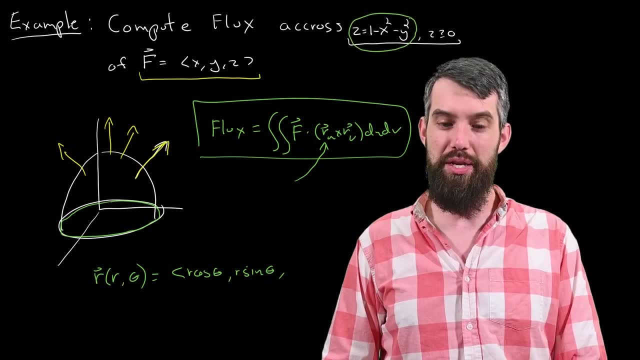 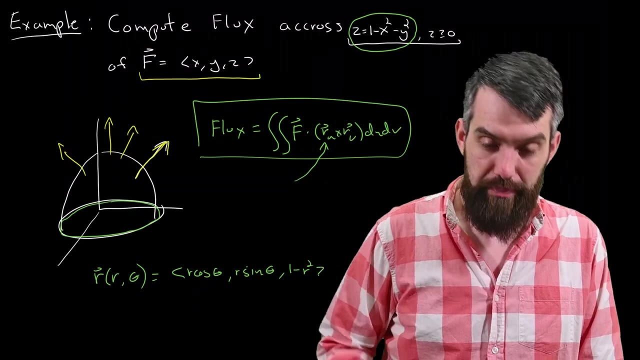 theta, The y component is r sine of theta. And then let's think about the z component. I know that z is 1 minus x squared, minus y squared. So in our theta coordinate, x squared plus y squared is r squared. So this is 1 minus r squared. So that's the surface, But I 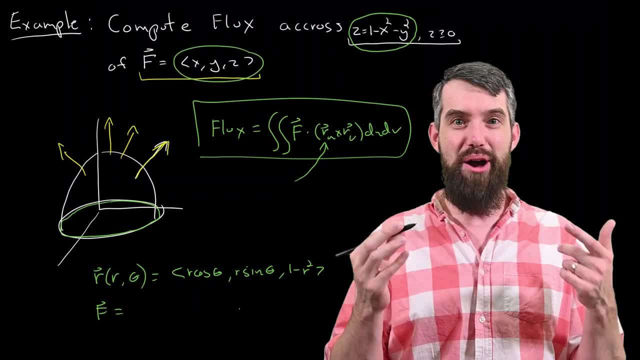 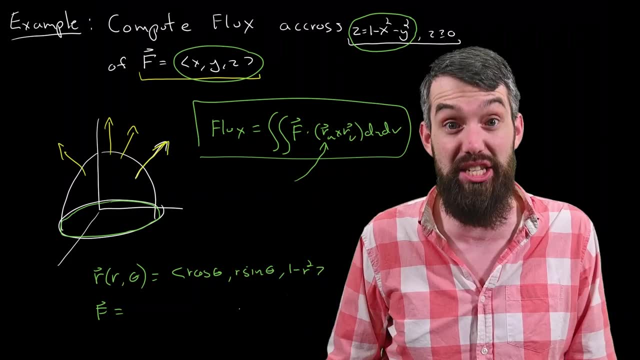 also have this field, which was x comma y comma z. Now it turns out that the choice of field that I have here, f being x y z, that just gives you the position. It's the same thing as the r There. 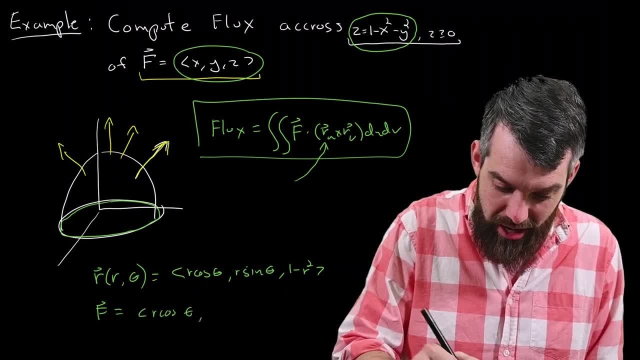 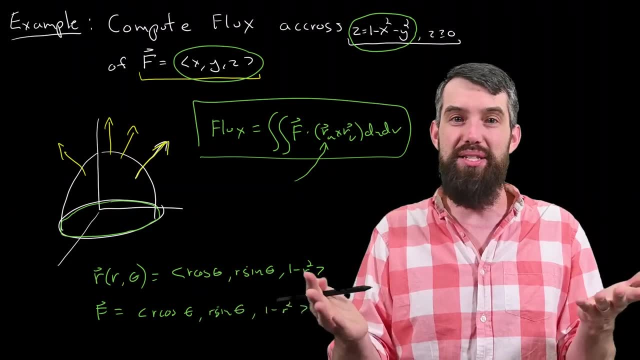 really is no difference. So this is just going to be r cosine of theta, r sine of theta and 1 minus r, squared, exactly the same as what we just had, And this is just a coincidence by the specific choice. Generally, if it was some other function, 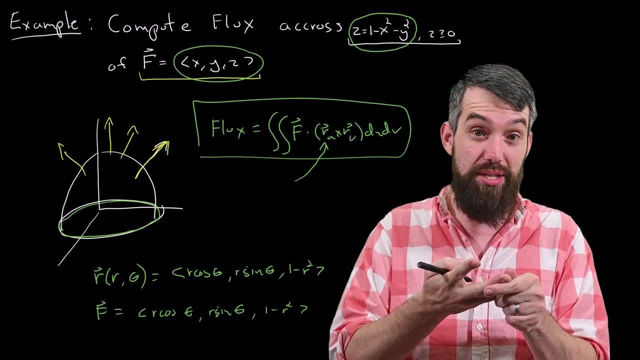 of x, y and z. you'd just plug in the r cosine of theta, the r sine of theta and the 1 minus r squared into whatever those functions were going to be. So that's the r and the f, But I do have. 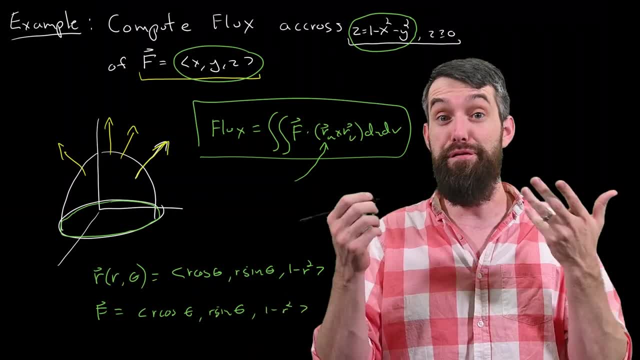 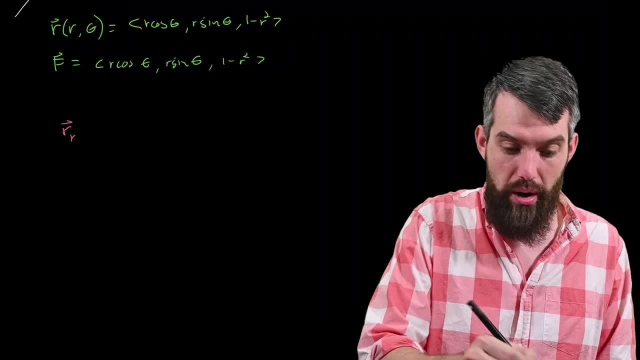 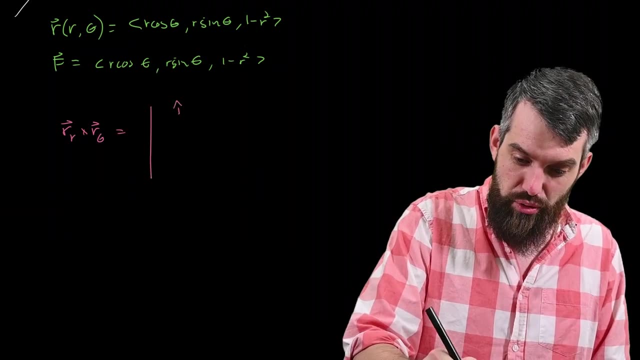 to compute the partial derivatives still and plug them into my formula, which is the cross product formula. Okay, so now I want to compute out: rr, the partial with respect to r, crossed r, theta, the partial with respect to theta. So I'm going to define, to be a determinant of this sort of funky matrix here, And I had to do some. 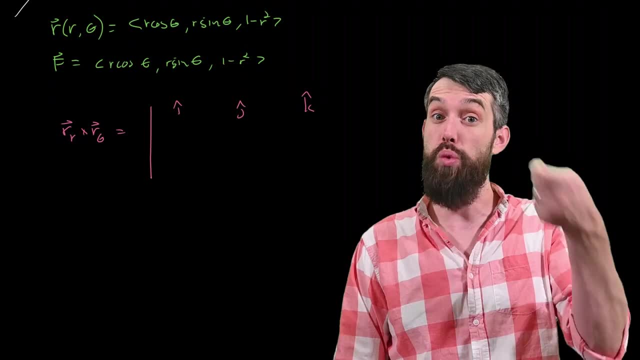 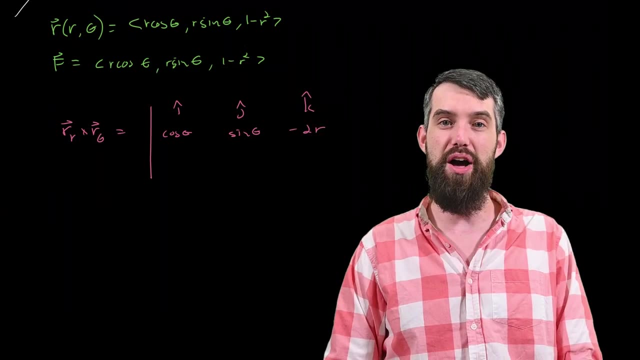 partials in my head here. So the second row is the partial with respect to r. So that's going to be cos, theta sine theta and minus 2r. the derivative of 1 minus r squared is minus 2r. 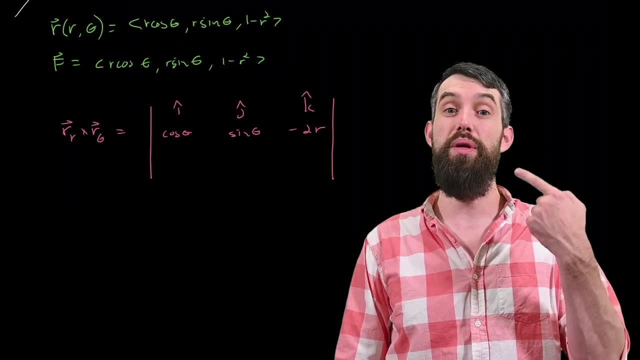 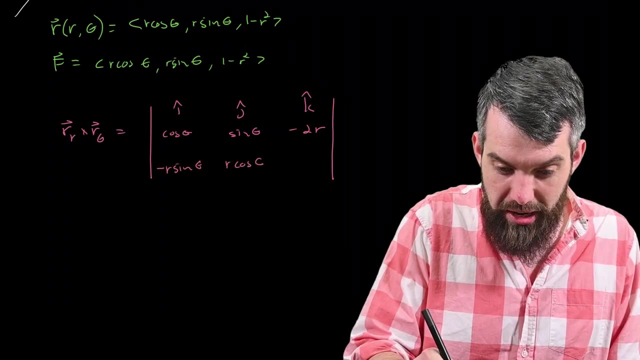 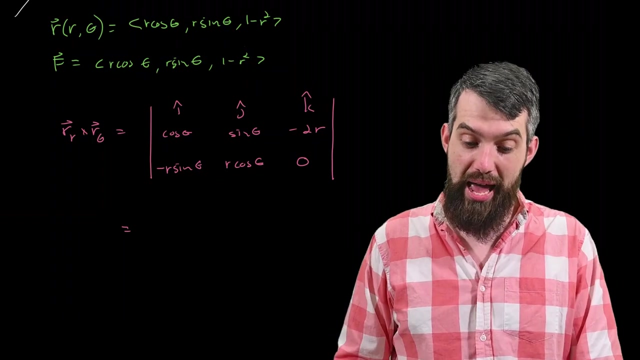 Then for the third line, this is the partial with respect to theta. So I'm going to take a minus r sine of theta and r cosine of theta, And then just a zero in that third component. This is straightforward to compute. So in the i-hat, 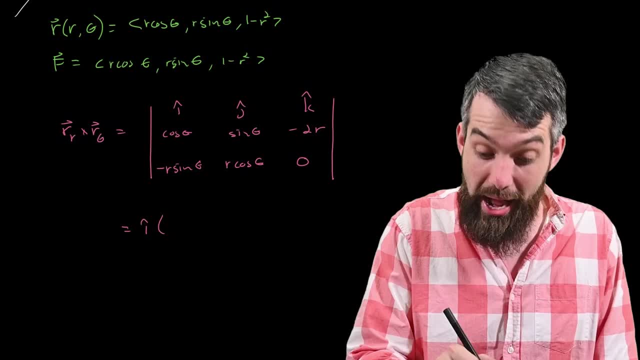 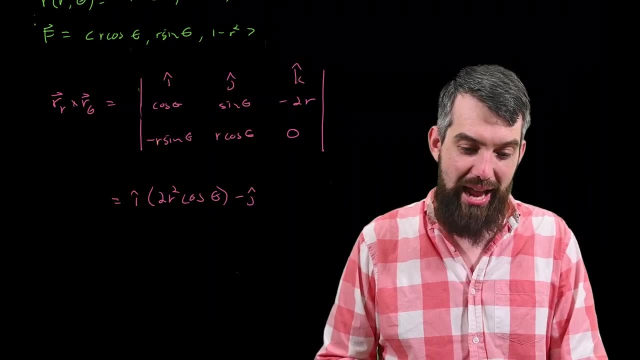 I'm going to have minus minus 2r squared cosine of theta. All right then I have a minus j-hat. It looks like a minus, minus, minus, which is three minuses, makes one minus. I have one there. 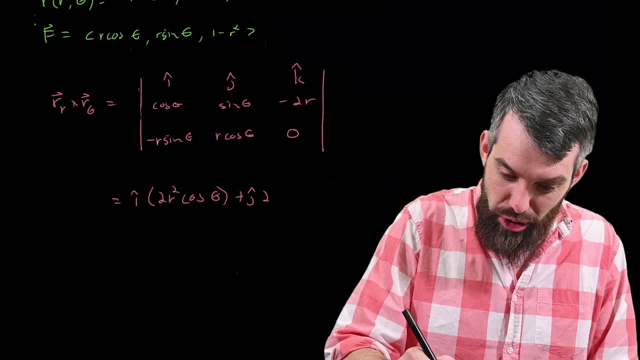 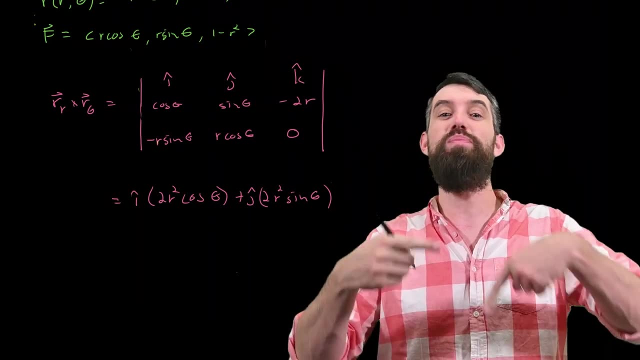 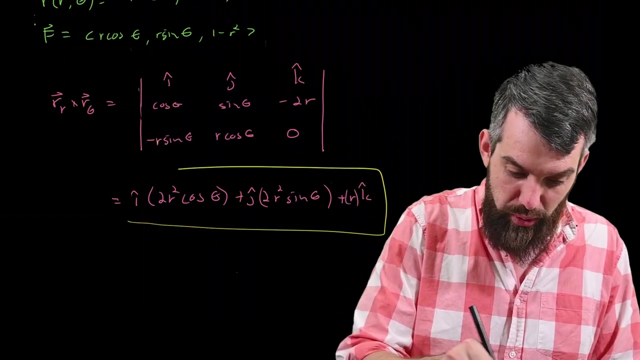 four minuses, lots of minuses, Anyways, of 2r squared sine of theta, And then finally, plus a k-hat times r cos squared, plus r sine squared, which is just plus r. So plus r times k-hat. Now, that was the cross product, which was one of the two things in my 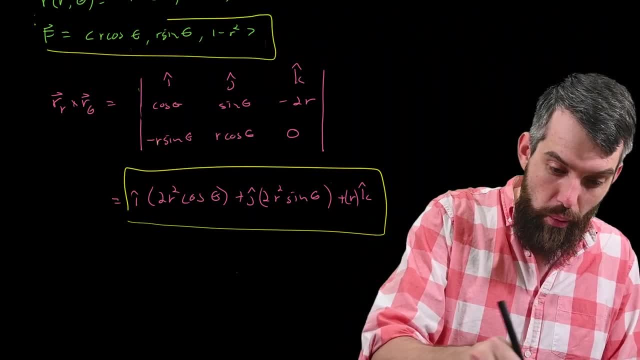 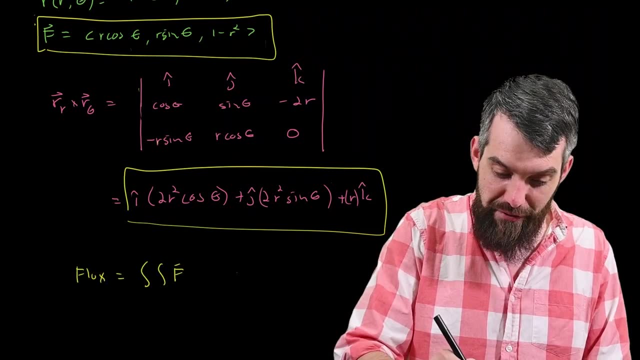 dot product of my original formula. The other was the field itself. So if I want to compute out the flux, which was the double interval of the f dotted with the rr, cross, r, theta, dr, and then I'm going to have the f dotted with the rr, cross, r theta, 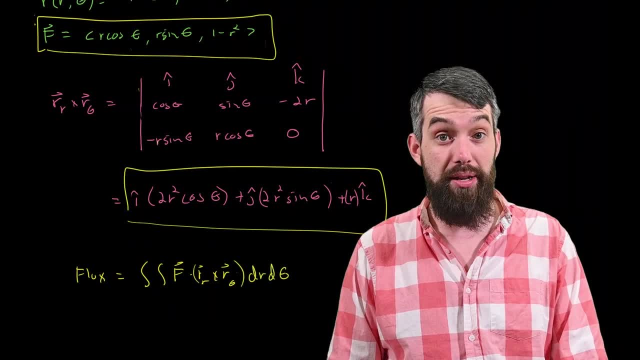 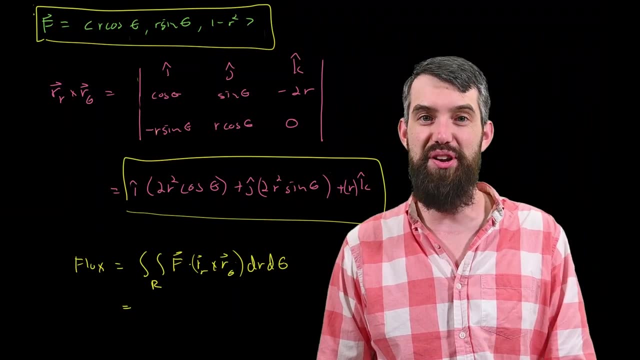 So if I want to compute out the flux which was the double interval of the f dotted with the rr, cross, r, theta, d, theta, well, I have to take the dot product of these two things that I've computed. Okay, so let's see if we can do that. I'll just put a big R down here for region, because I haven't. 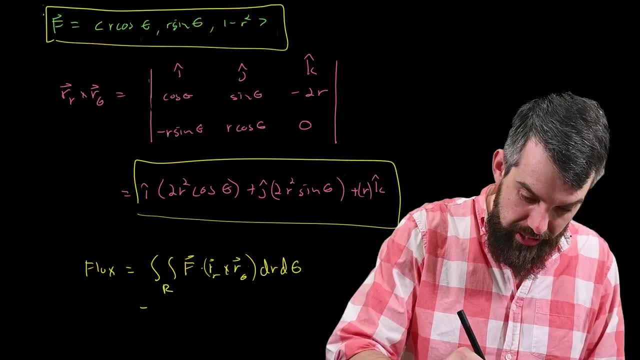 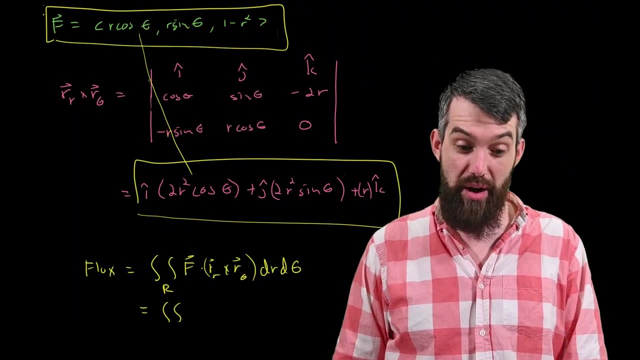 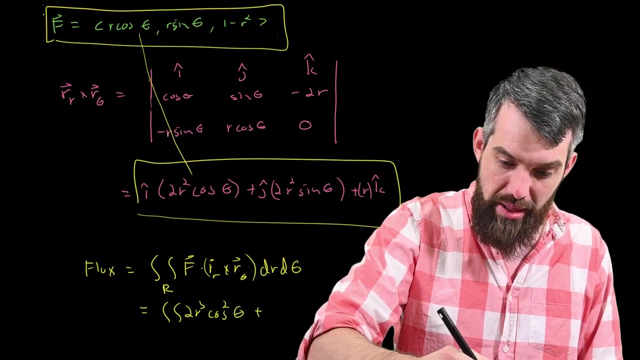 figured out my limits of integration yet I'll do that shortly. Anyways, this is a double interval. And then my f dot dr. well, it's sort of the first component there and the first component there multiplied together, So I have a 2. looks like r cubed cos squared theta. Then the second.